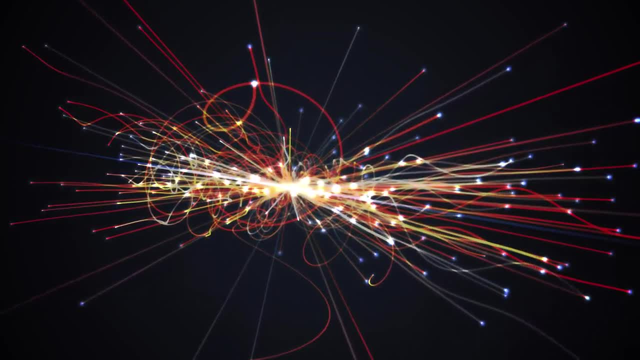 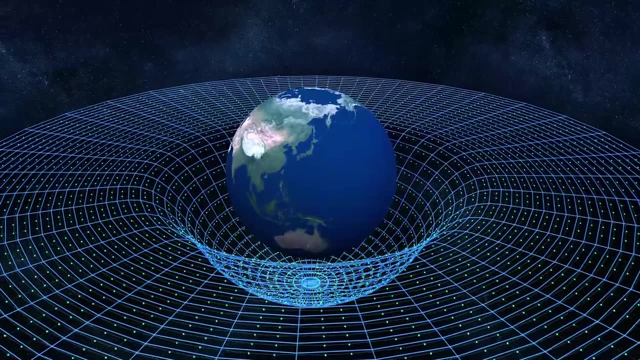 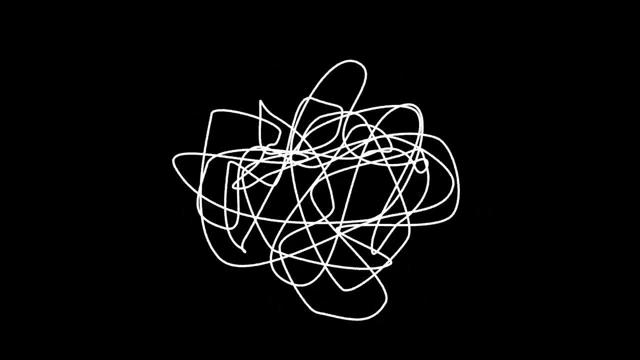 particles collide, they get an endless amount of energy crammed into a small space. One probable solution that theorists acquired from nuclear physicists in the 1970s was to abandon the complex point-like gravitation particles. Strings are capable of colliding and rebounding without implying physically impossible infinities. 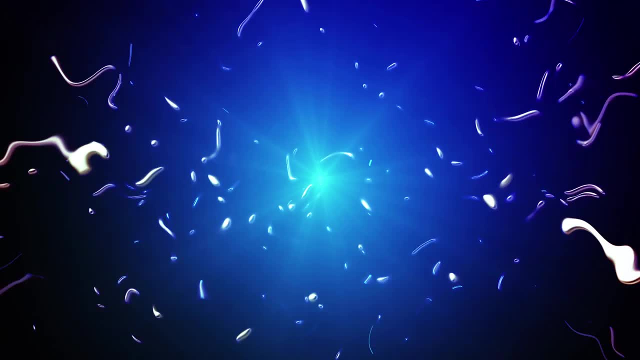 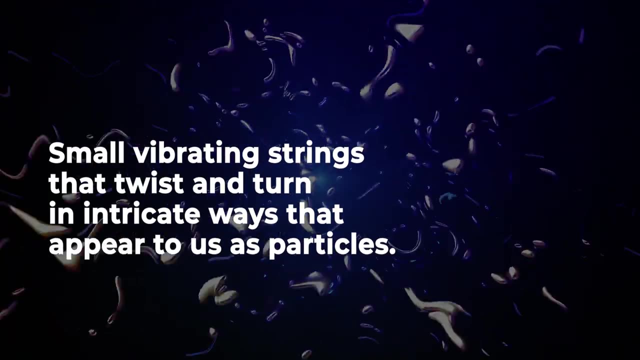 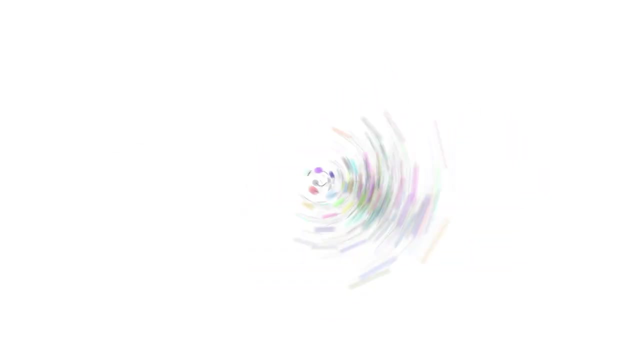 String theory rewrites the traditional universe description by replacing all matter and force- particles- with only one element: small vibrating strings that twist and turn in intricate ways that appear to us as particles. A photon may be formed by a string of a specific length, striking a specific note and a quark. 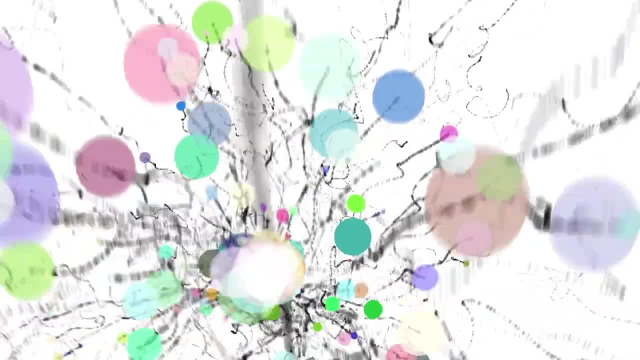 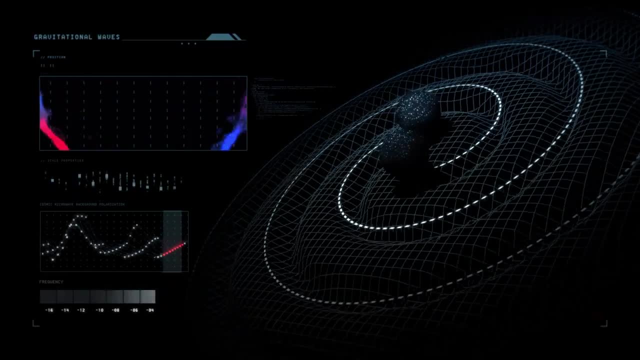 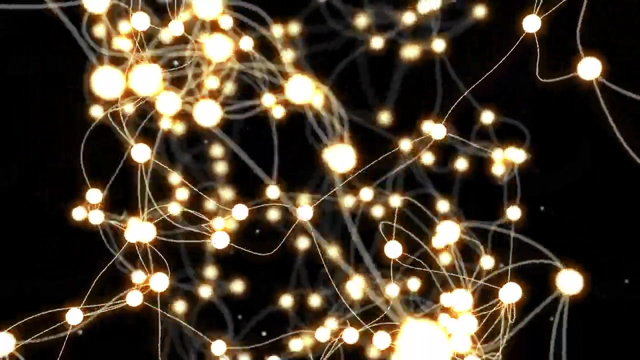 could be formed by a string folded and vibrating at a different frequency, and so on. Besides taming gravity, string theory was appealing because it promised to explain supposed fundamental constants like an electron's mass. Theorists hoped that the next step would be to find the appropriate 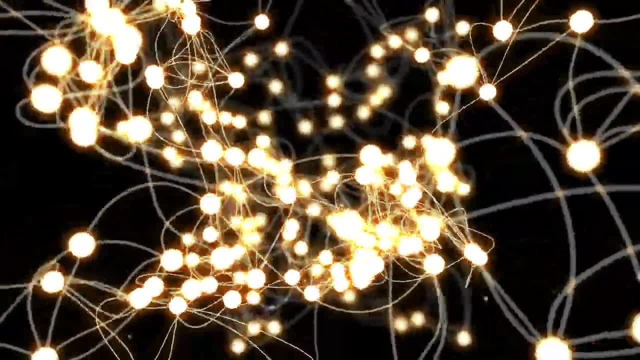 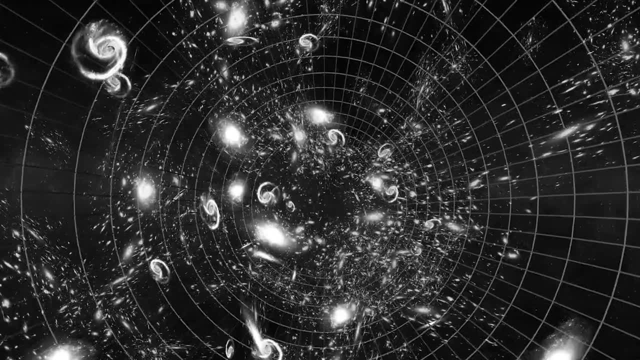 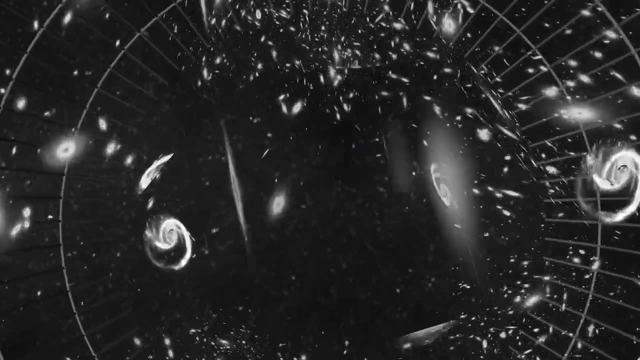 way to explain the folding and movement of strings. then everything else would follow. However, that early simplicity came at the expense of unexpected complications. String math didn't operate in our four-dimensional world, that is three of space and one of time. 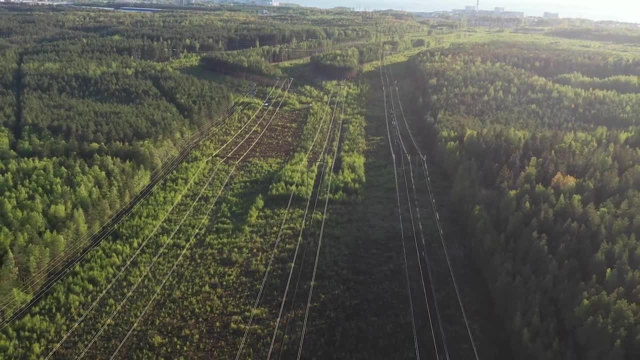 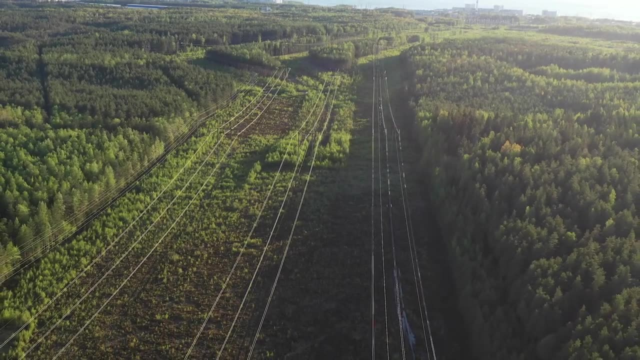 It required a total of ten dimensions, six of which were visible only from the perspective of the small strings. similar to how a power line appears as a 1D line to birds flying far overhead but looks like a 3D cylinder to an ant crawling on the wire. 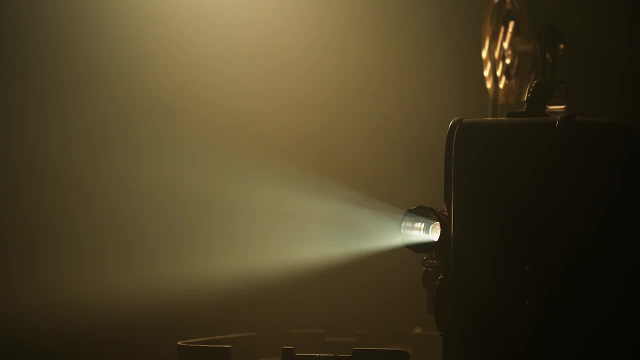 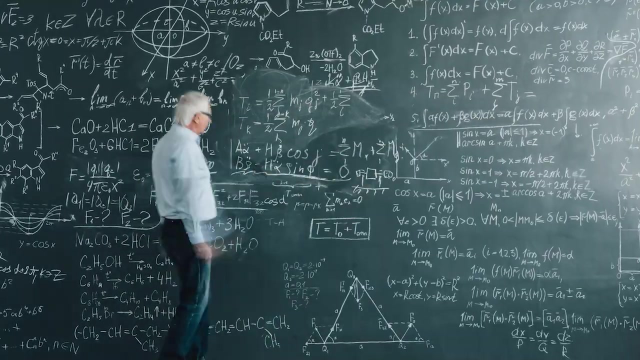 Today's string theory differs significantly from that of the 1960s and 70s. Researchers are divided on whether it is still the best candidate for a theory of everything with adjustments, or whether theorists should forsake it in favor of other subjects. 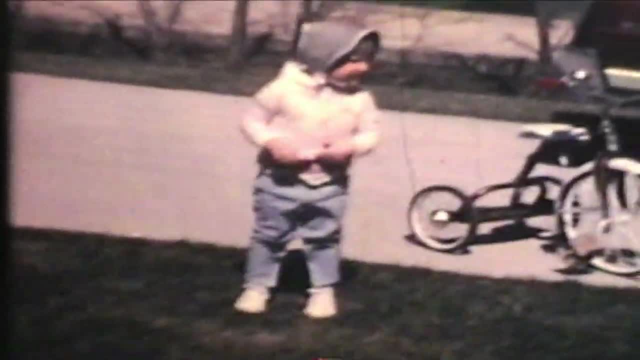 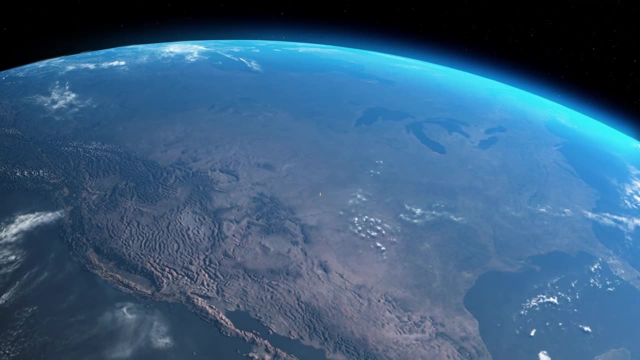 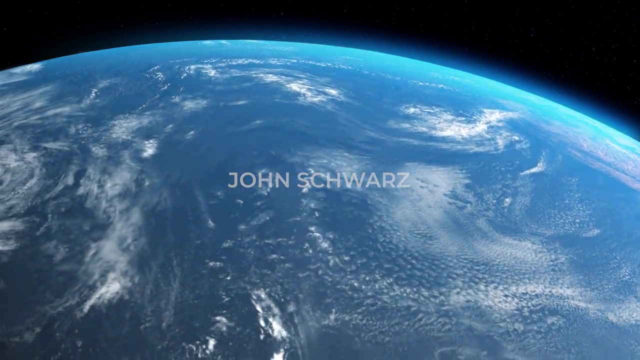 There were several solid reasons to bring a standstill on working on the string theory between 1973 and 1974. It remained negligible for many years until the string theory revolution in 1984, when theoreticians Michael Green and John Schwartz came up with equations.